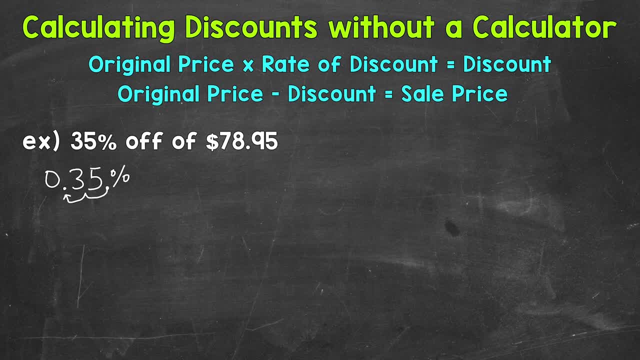 we take our original price, $78.95, multiply it by that rate of discount in decimal form. So let's write that out: $78.95 times 35% in decimal form, So 0.35.. So let's calculate that And I'm going to come to the right in order to go. 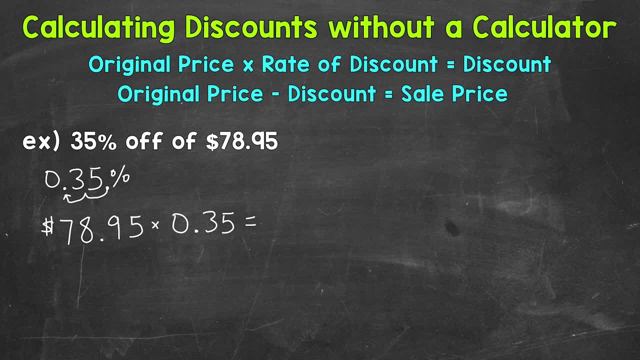 through those steps. Now, when we multiply decimals, we can take the decimals out and then place the decimal in the answer once we get to that point. So I'm going to take the decimals out and multiply 7,, 8,, 9,, 5 times 35. And again, we will worry about the decimal at the end. 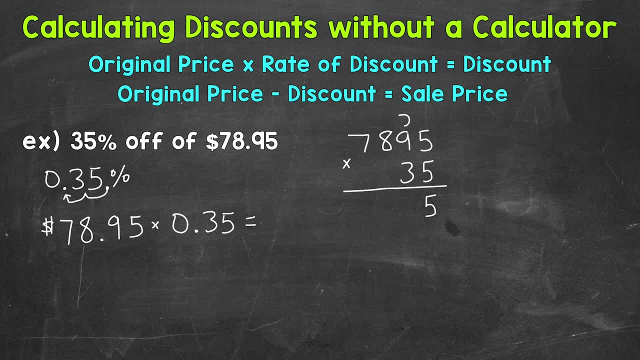 5 times 5 is 25.. 5 times 9 is 45 plus 2 is 47.. 5 times 8 is 40 plus 2 is 47.. 4 is 44. And then 5 times 7 is 35 plus 4 is 39. We are done with this. 5.. And then the 2,, 4, and 4.. 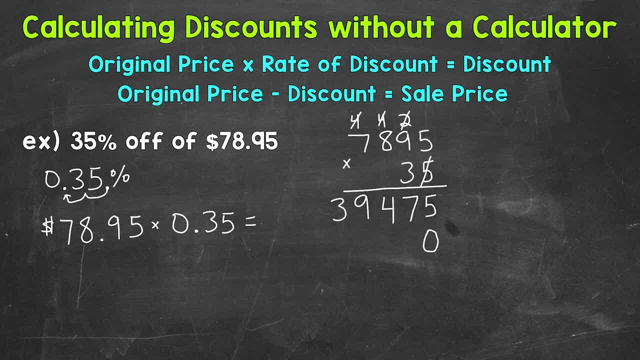 We need our placeholder 0 because we are moving one place value to the left. And now we can do 3 times 5,, which is 15.. 3 times 9 is 27 plus 1 is 28.. 3 times 8 is 24 plus 2 is 26.. And then 3 times 7 is 21 plus 2 is 23.. 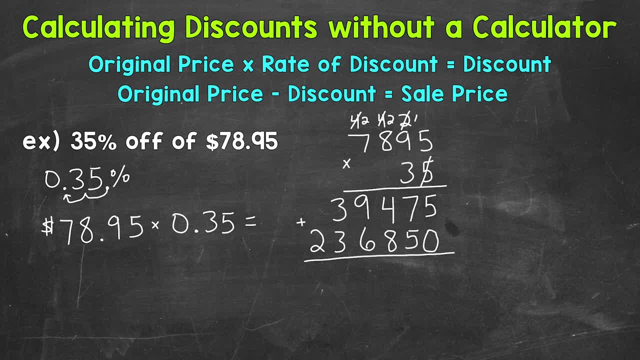 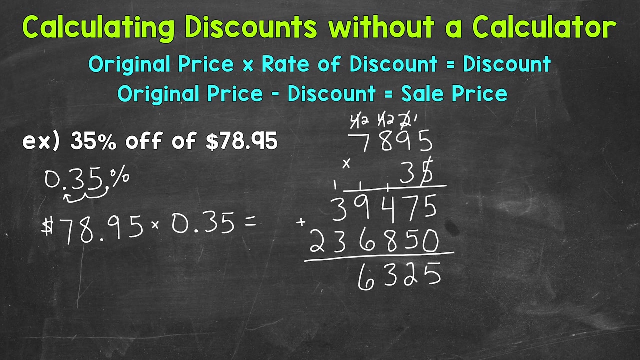 So now we add here: 5 plus 0 is 5.. 7 plus 5 is 12.. 1 plus 4 is 5 plus 8 is 13.. 1 plus 9 is 10 plus 6 is 16.. 1 plus 3 is 4 plus 3 is 7.. And then we have a 2.. 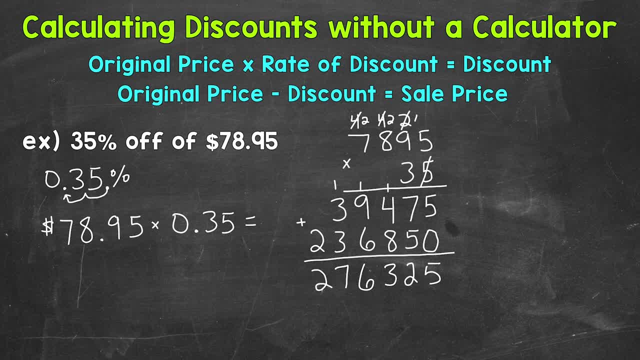 So now we're ready to place our decimal, So we look back at the original problem and see how many digits are to the right of a decimal or how many digits are behind a decimal. Well, we have 1,, 2,, 3,, 4.. So that's how many digits are going to be to the right of the decimal in our answer. 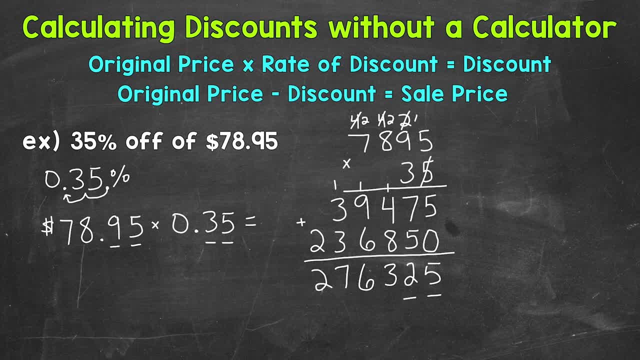 So we can count off 1,, 2,, 3, 4 digits. Our decimal is going to be placed in between the 7 and the 6.. So we get- let me rewrite this without the lines underneath- So we get 27.. 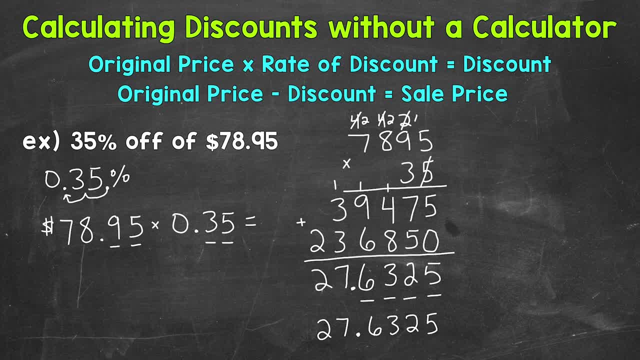 6, 3,, 2, 5.. Now we are working with money, So we need to round this to the hundredths place. We have a 3 in the hundredths place. Look at the digit to the right. We have a 2.. 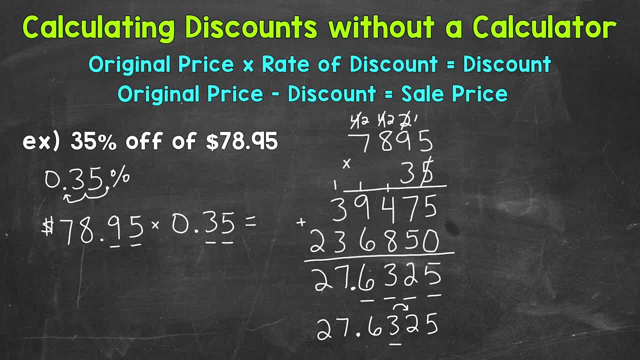 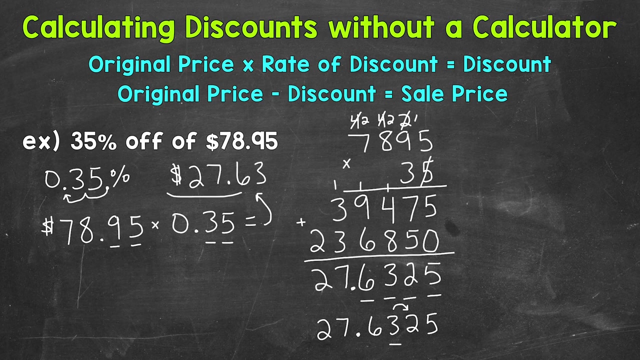 That 2 says we stay the same. So we are going to get $27.63.. So $78.95 times 0.35.. I ran out of room here so I'm going to write it above. That gives us $27.63.. So that's our discount. That's how much money we are taking off the. 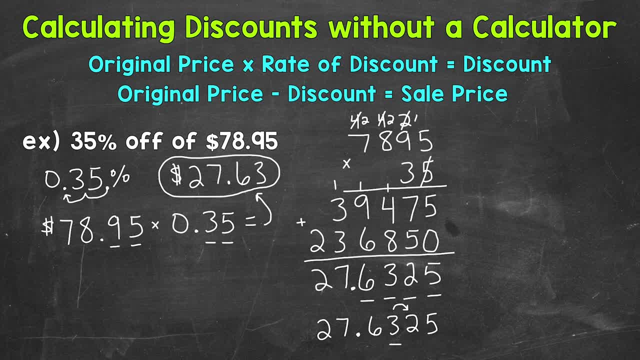 original price, That's 35% of $78.95.. So once we have that information we can subtract that discount from the original price. So the original price minus the discount, We are taking the discount off of the original price. The original price. 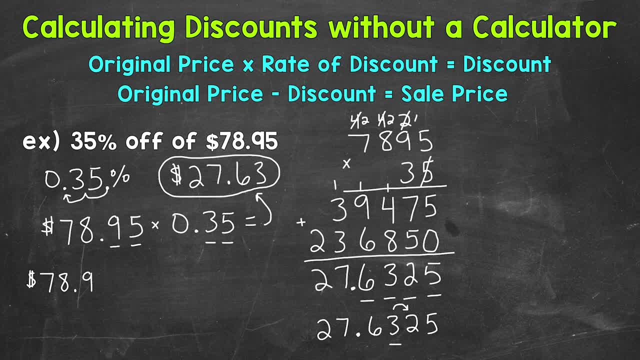 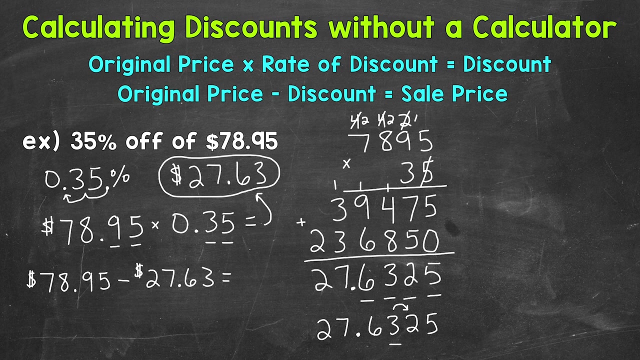 $78.95. And we are subtracting $27.63.. So let's see what our sale price is going to be. Now, when we subtract decimals, we need to line the decimals up. So I'm going to calculate this to the right. So we have $78.95 minus $27.63.. So the decimals are lined up and that's going to.